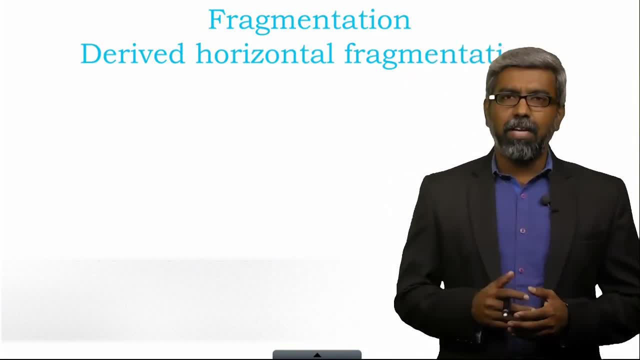 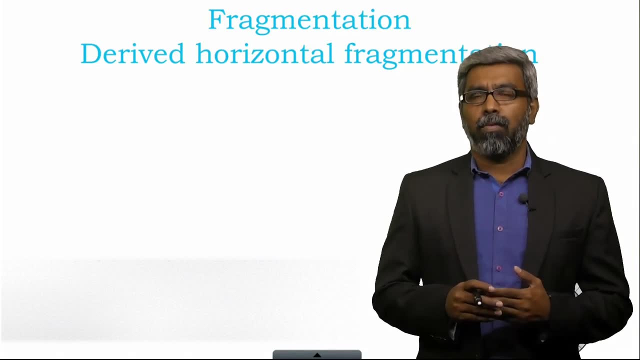 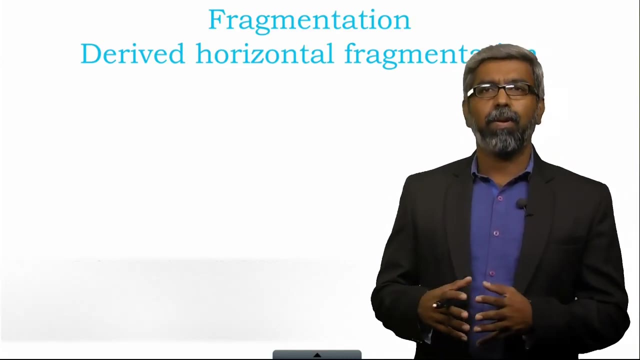 they are related to other relations and that relation is through the primary key and the foreign key relationship. We usually call the primary key table as the parent table and the foreign key table as the child table. So the primary key which is in one table. 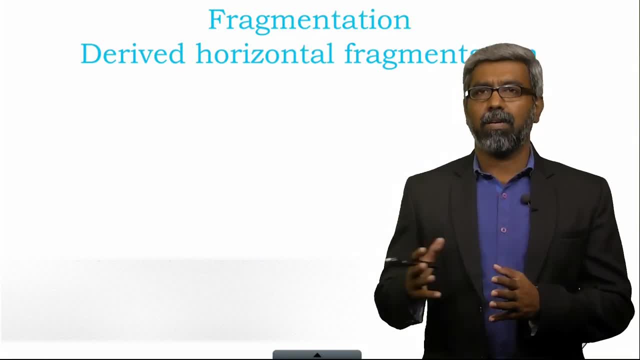 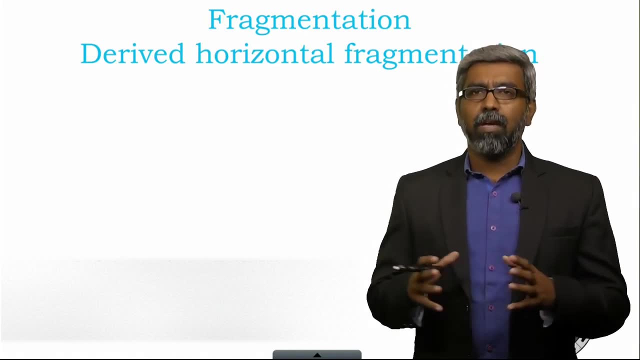 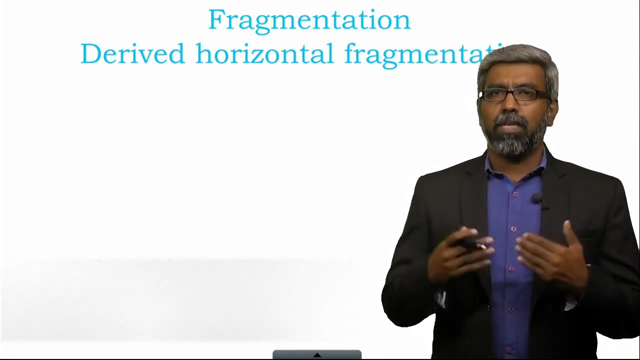 the same attribute is included in the another table as a foreign key, So it is going to refer. that is, the domain of these two are going to be same and we establish link between these two tables: the primary key and foreign key. Now the question is so when we derive, there is when we go for primary, horizontal fragmentation- 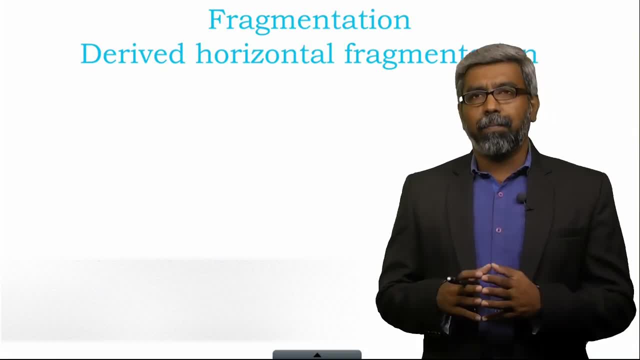 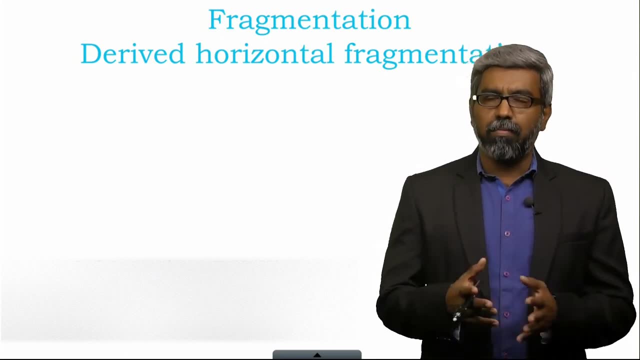 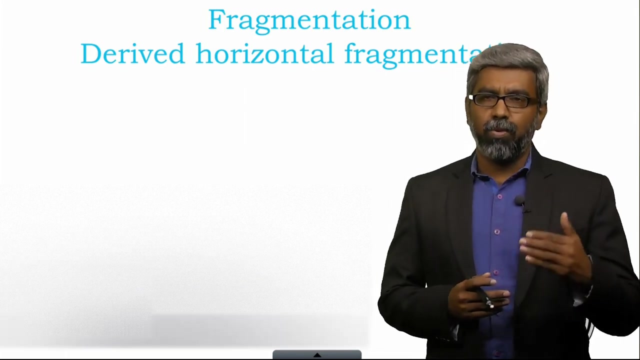 we consider just one table And in reality I cannot fragment all the individual tables using the Set of minimum predicates we have derived. minimum fragment: we have derived. it is a difficult task. The reason is, if I fragment one table on set of attribute values, on set of attribute. 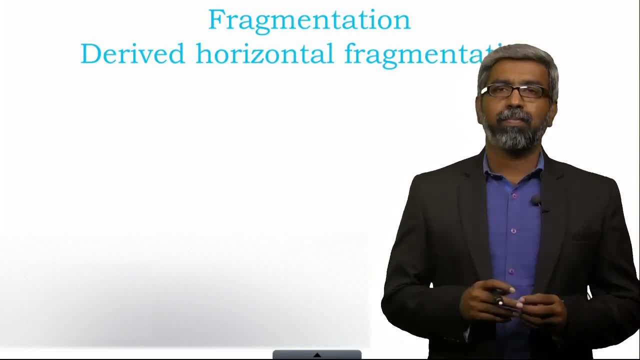 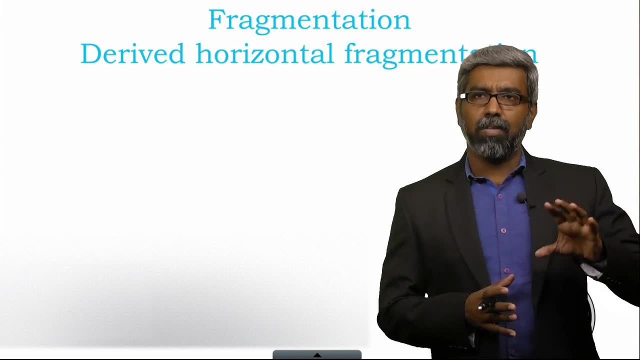 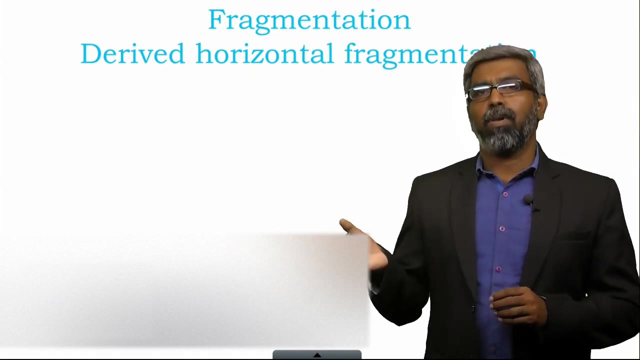 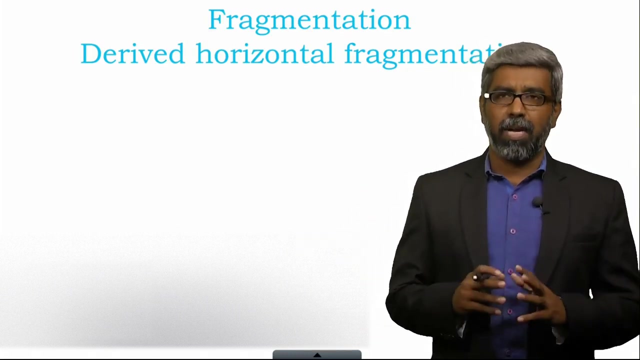 the same set of attribute may not present in other tables. Now the question is: how do we fragment the other tables? because if we send, for example, a student personal data to one particular site and the marked data stored in a different table and we must send the student marked data to the same site. So how do we do that? 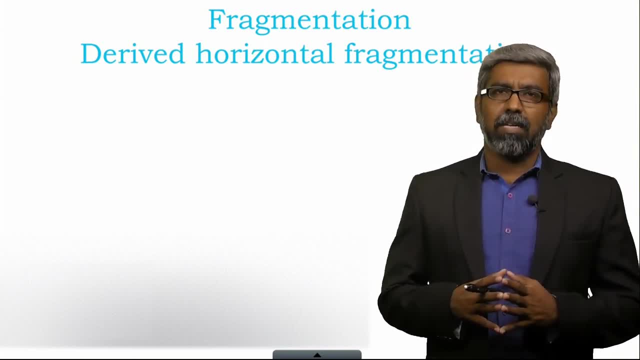 So for that process we call these fragments as derived horizontal fragmentation. So the another variety of Horizontal Fragmentation is derived Horizontal Fragmentation. Let us discuss about the derived Horizontal Fragmentation in this class Now. I am going to go through an example now. So let us see how we can help you to derive. 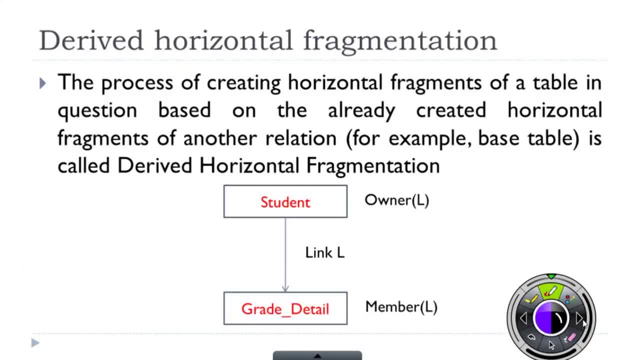 this lecture. Now let us go to the presentation. Derived horizontal fragmentation is the process of creating horizontal fragments of a table in costin based on the already created horizontal fragment of another relation, For example the base table. this is called the derived. 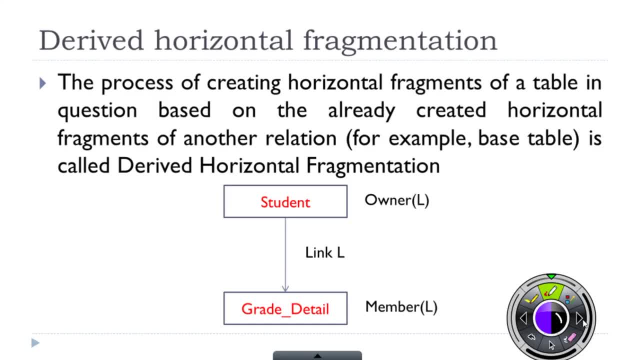 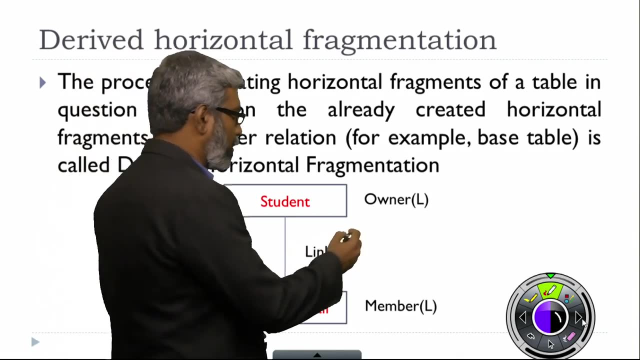 horizontal fragmentation. So when I have a database, so relation one relation is linked with other relation through the foreign key, primary key, primary key, foreign key relationship. So we can, we may call that table with the primary key as the owner relation primary. 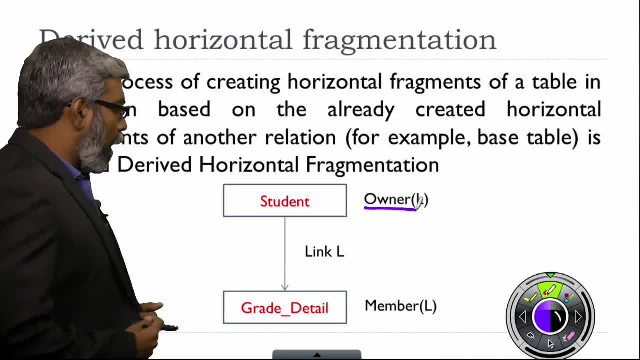 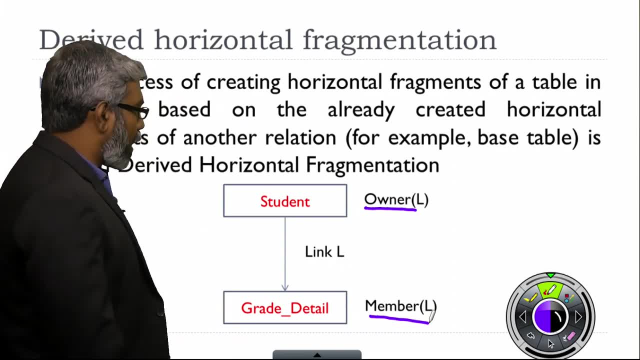 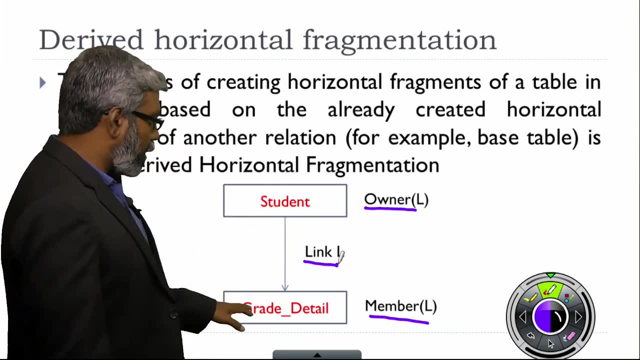 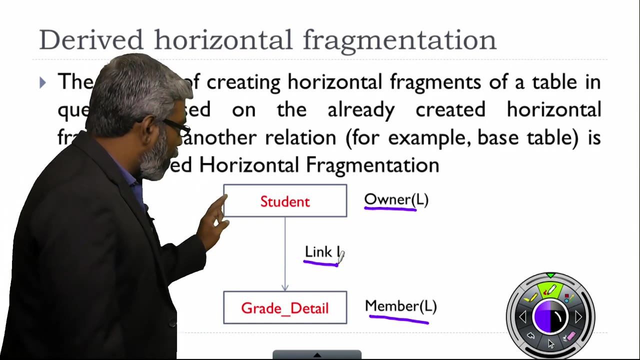 key as a owner relation and the foreign key table as the member relation. Now there is a link that connects these two tables. So we have a primary key in the owner relation and the foreign key in the member relation. Here the domain of the primary key attribute of owner table and the foreign key attribute. 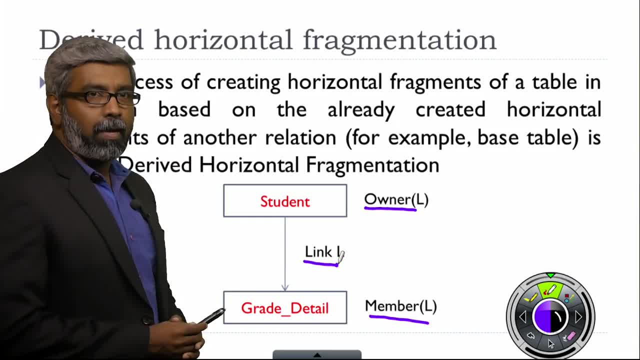 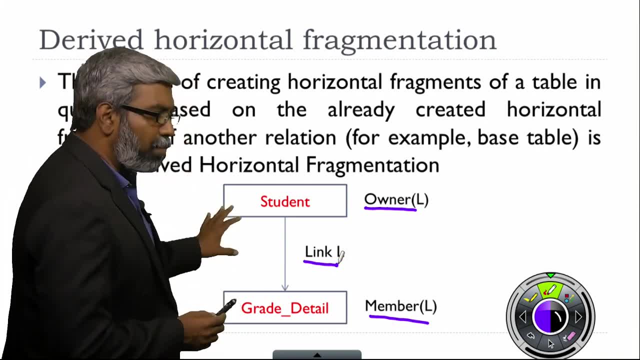 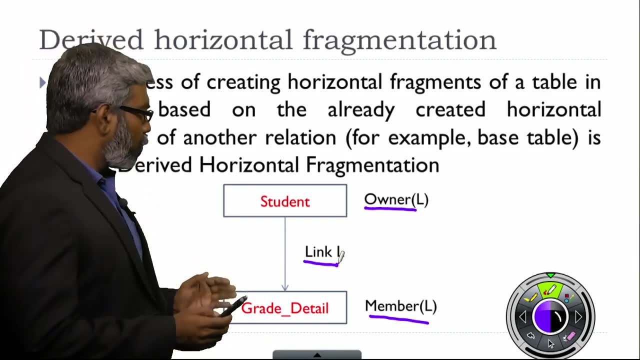 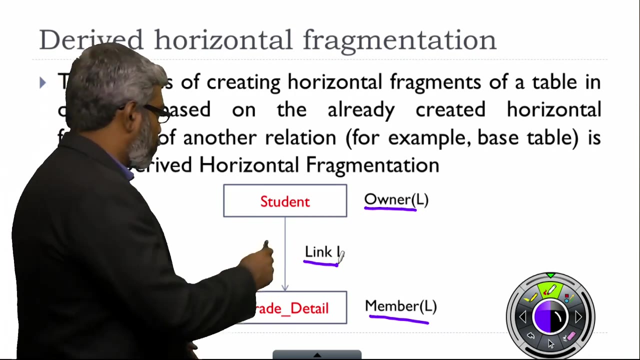 of member table are going to be same. So now the idea is I am going to fragment one of these tables using primary horizontal fragmentation and the other one using derived horizontal fragmentation. So which is the table? So let us for example these two tables- student, as well as the grade, detail both. 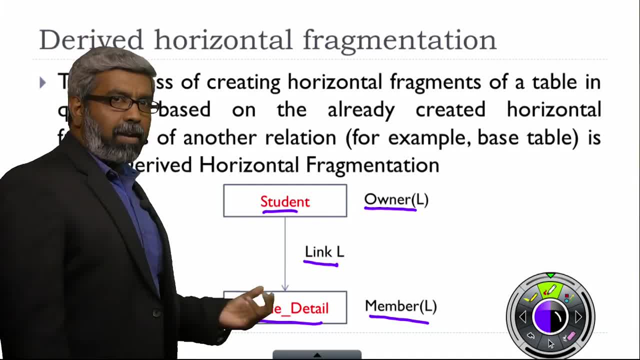 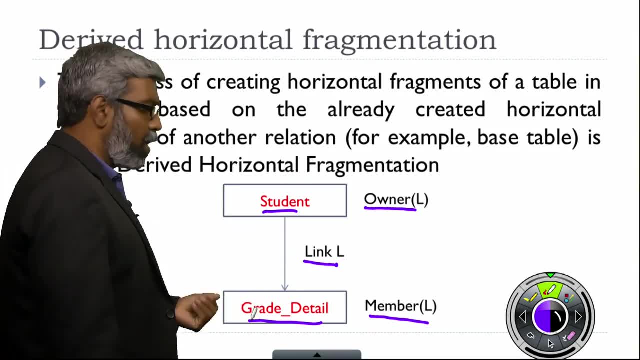 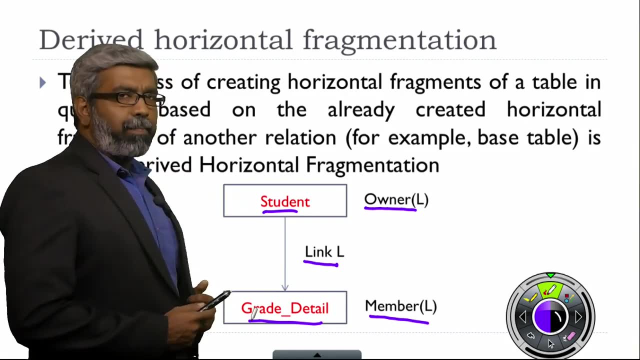 the tables are going to share an attribute which is common in domain, which is common in domain of permitted value: the permitted value stored in these two tables. Now we take the primary table, that is, the table with the primary key, and we fragment. 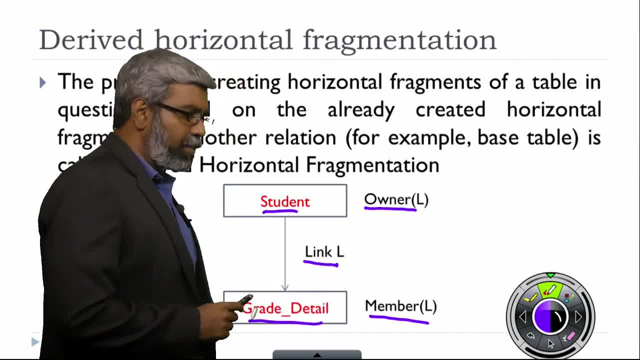 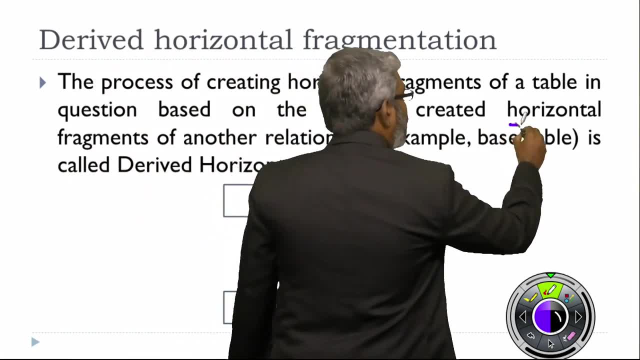 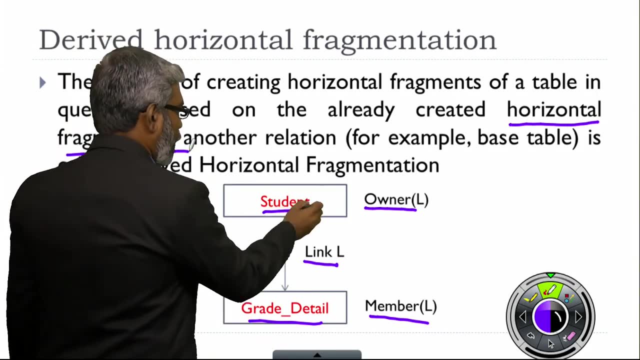 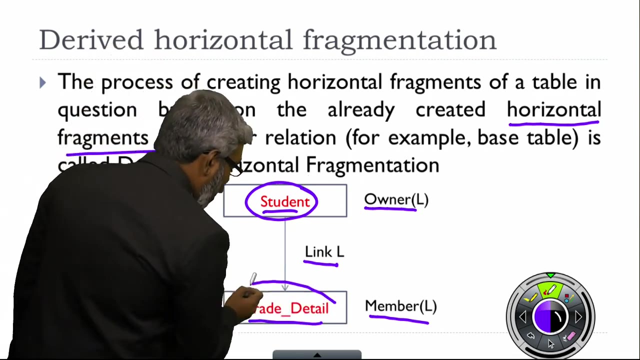 the table using Primary horizontal fragmentation. then we use the fragments. we use the horizontal fragments that were created from the student relation, from the student relation to further fragment the member relation. that is, in our case, the grade detail. Semi-joint is a joint operation. 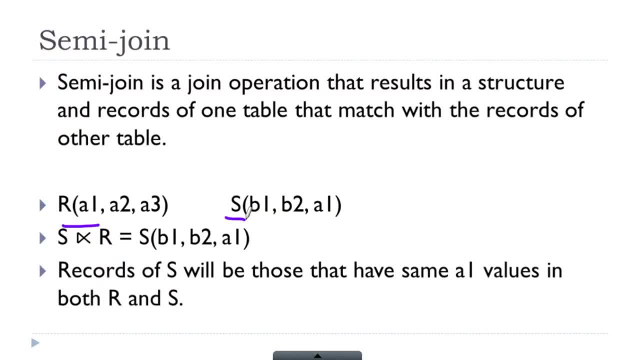 that results in a fragmentation. Semi-joint is a joint operation. Semi-joint is a joint operation. So we have two tables, the tables in a structure, and records of one table that match with the records of the other table. So here you see, we have two relations. One is R, the other 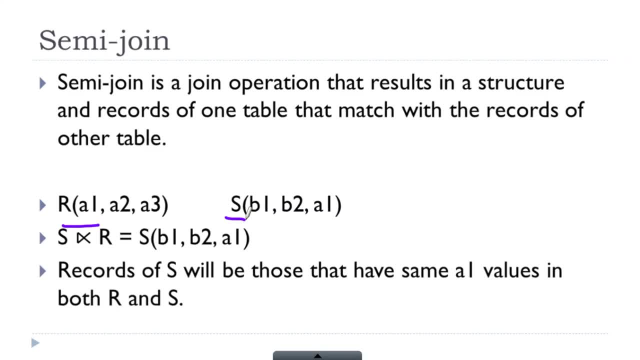 one is S. R has three attributes: a1, a2, a3,. S has three attributes: b1, b2 and a1.. If you observe this from these two tables, you can understand. a1 is the attribute which is common between these two tables. 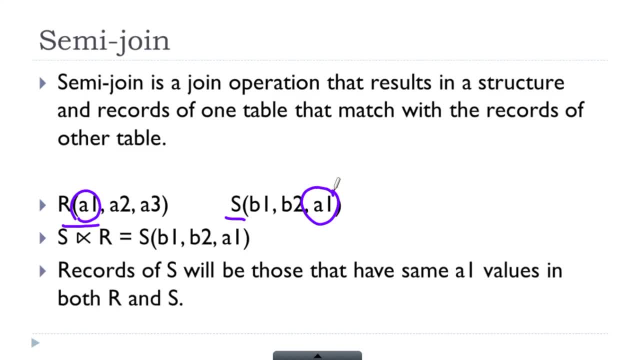 in many cases the name may be same or may be different, But the thing is the domain of this attribute and the domain of A1 in S. both are same. Now the symbol is: this symbol is the semi-joint symbol, So S semi-joint R is equal to. I will get the structure of S alone. You. 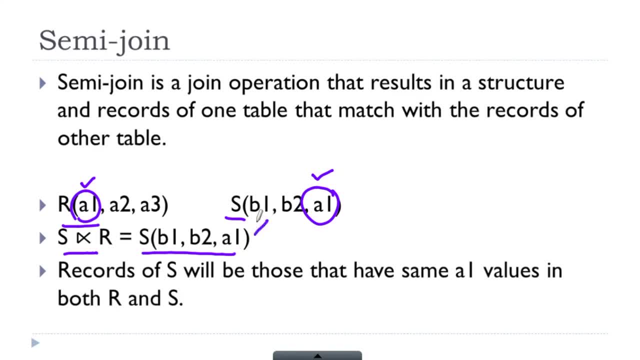 observe carefully, See, it looks like S as it is, without any changes. So no attribute is taken from the relation R. So this is semi-joint. But what about records? The records are filtered. Records are filtered on comparison of A1 of table S with A1 of table R If both values are same. 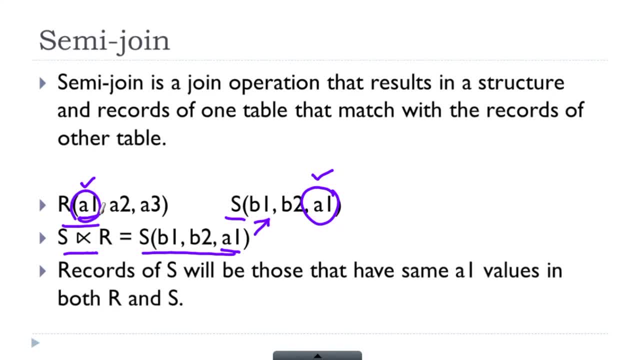 they are same. If both values are same, they are same. If both values are same, they are same. That record will be included in this fragment. So S semi-joint R. see that the semi-joint it is open on the right-hand side. That means we do not take. 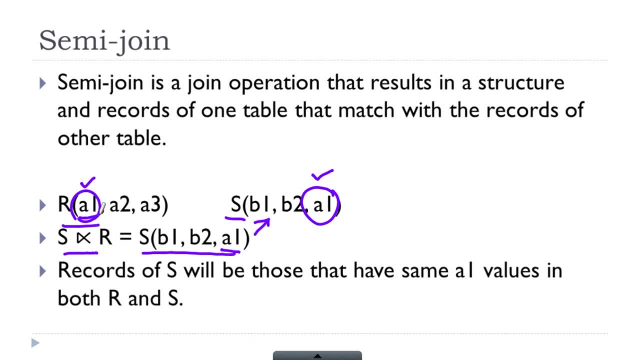 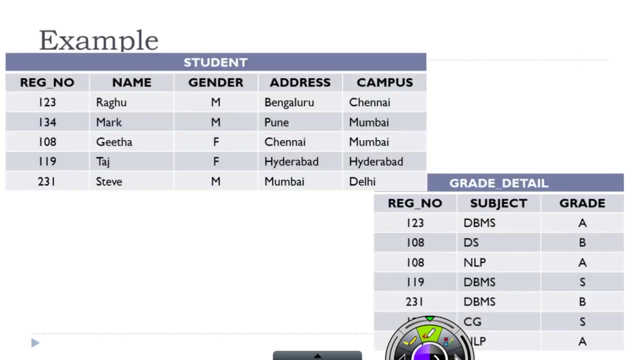 attributes from the right-hand side table. We take all attributes from left-hand side table. So this results in: records of S will be those that have same A1 values in both R and S. Now let us see an example this table: We have student table. 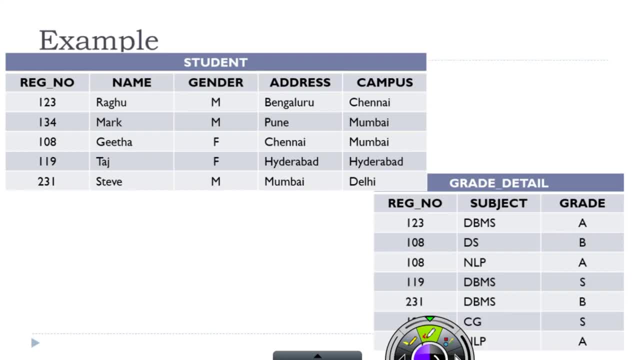 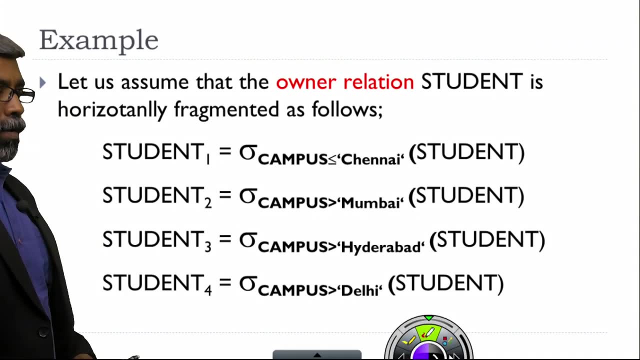 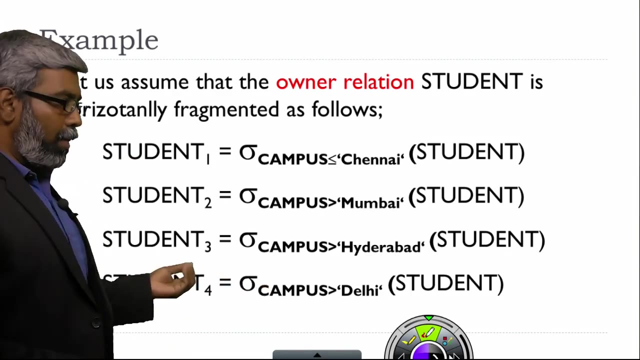 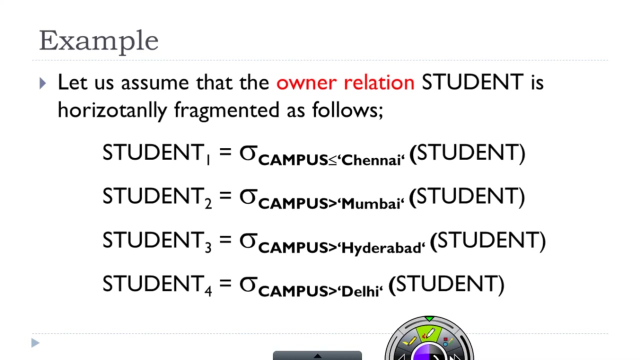 with some records and we have grade tables with some records. Let us assume that the owner relation- student- is already horizontally fragmented, horizontally fragmented on the campus attribute of student relation And the values chosen are Chennai, Mumbai, Hyderabad and Delhi. That means we have 4 different sites at each of these locations because we have 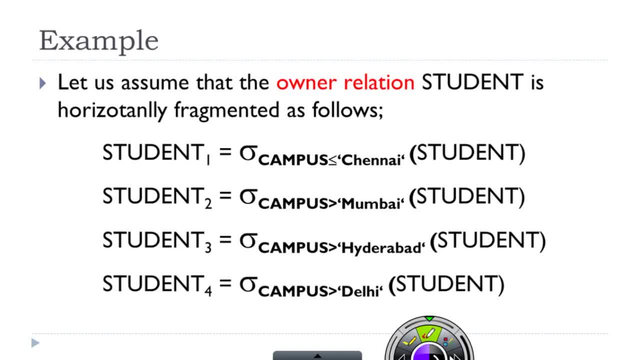 campuses in these locations. We have a campus in Chennai, we have a campus in Mumbai, Hyderabad and Delhi. That means we have already assumed that we have already fragmented the student relation according to this fragment, that is, min-term predicate and min-term fragment value. 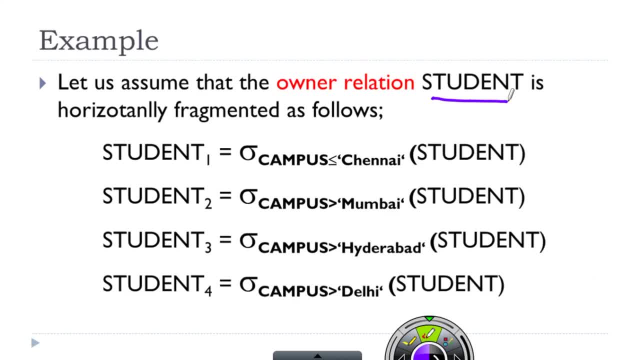 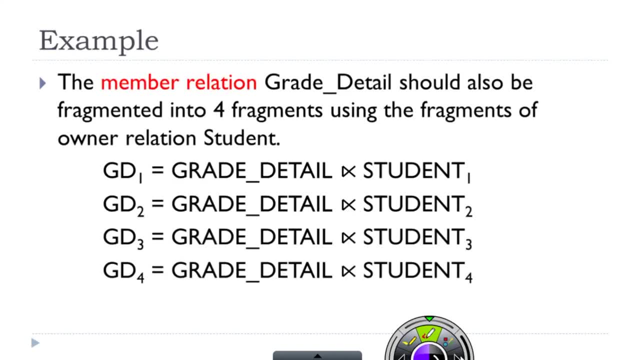 Campus is mobilehenheit. Now what we have is student one, student two, student three and student four. Now, if I am going to join this table, the member relation grade detail should also be fragmented into four fragments only because the primary table, that is, primary key table, student- is already fragmented, and into four fragments. So 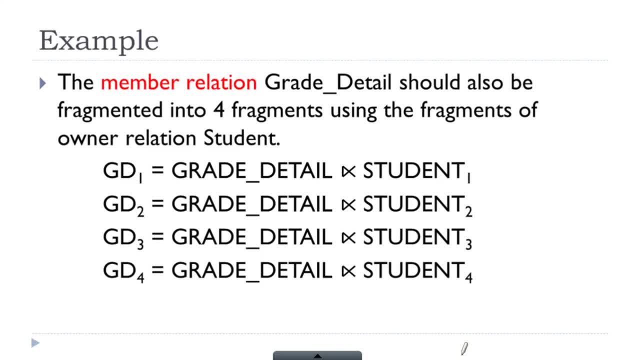 what we expect is, we want to fragment the member relation in such a way that the records related to those 4 already fragmented tables will end up in the same fragment, that is, same site. So that is where we are applying the semi-join operation. So how did we apply the semi-join? 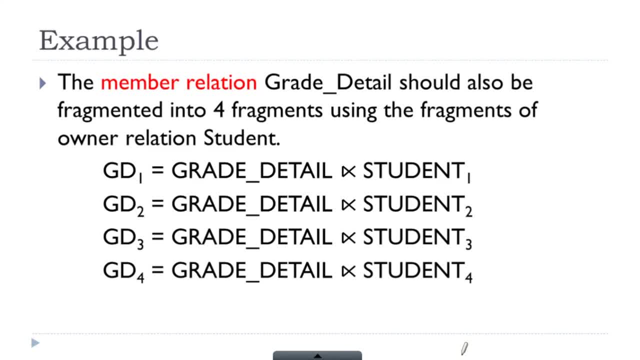 operation. So we create gray detail 1,. gray detail 1, by performing the semi-join between gray detail and student table, student 1.. Student 1 is the fragment that is that was resulted from the applying the minterm predicates, predicate 1.. Likewise, GD2, the same gray detail table. 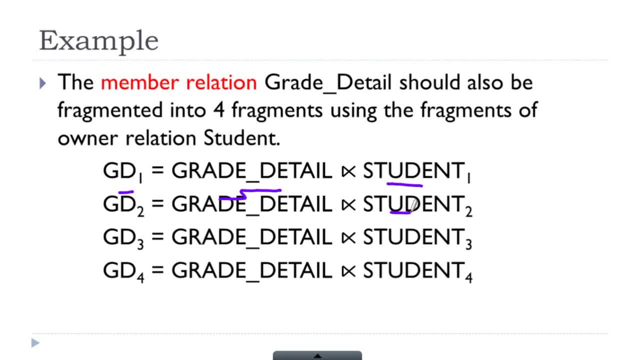 is semi-join with student 1.. So now what happens? Student 1 have. assume that student 1 have 10 records, grade detail. have all the records of it. Now the common attribute value, in our case the student register. 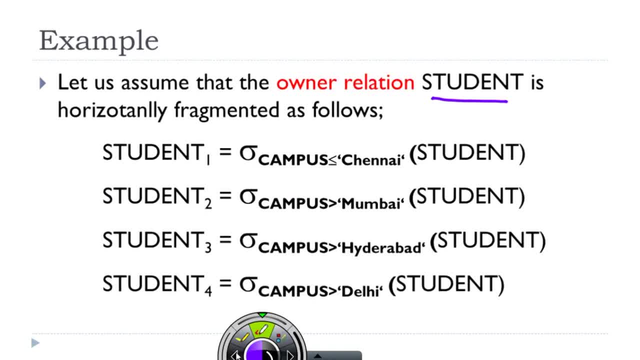 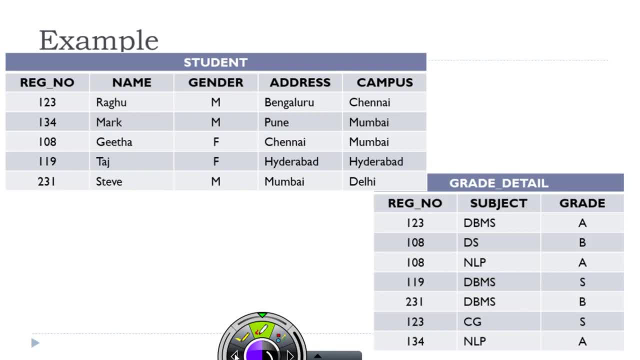 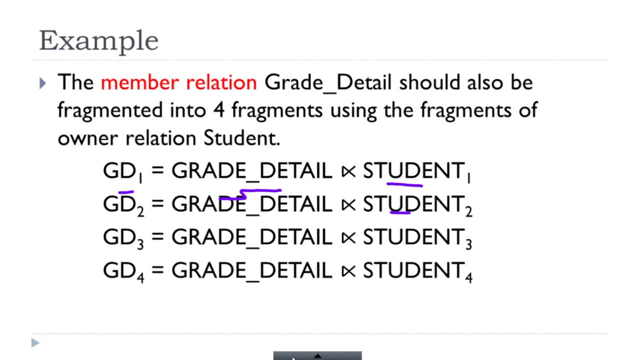 number is matched with. See here. register number of the student is common in both relations in student and grade detail And these two are compared. So the records of student 1 and grade details are compared on the value of the register number attribute. So only. 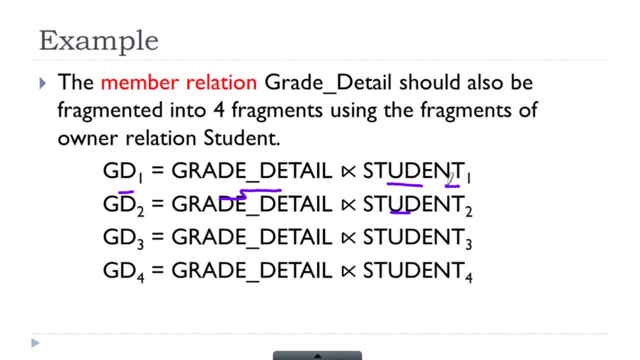 the register number of student 1 will match with the register number of the grade detail. So what we have- The fragment of the register number of student 1 and grade detail is according to the register number of student 1.. That is now student. 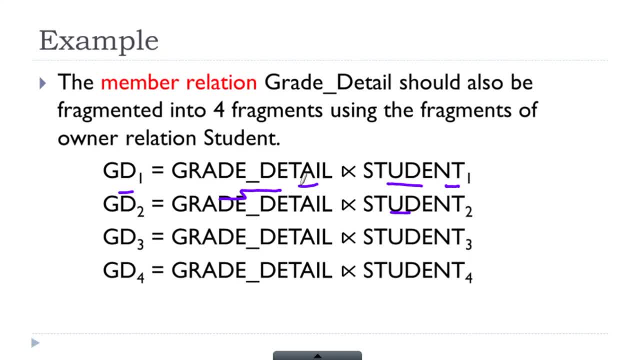 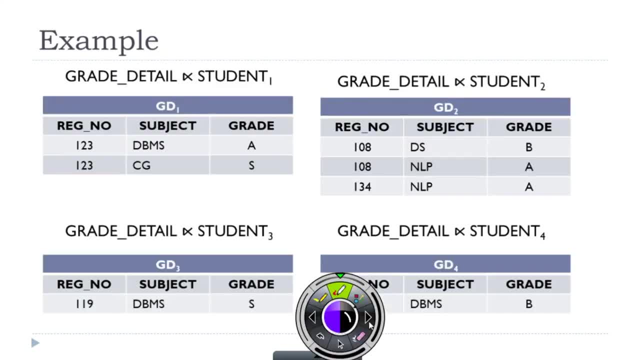 1 and GD 1 will have the records of same person, same set of people. So that is the idea of this derived horizontal fragmentation. See example here. what did we do? So? grade detail, semi-joint, student 1, it is end up in 2 records. 2 records Now the idea is the student 1. 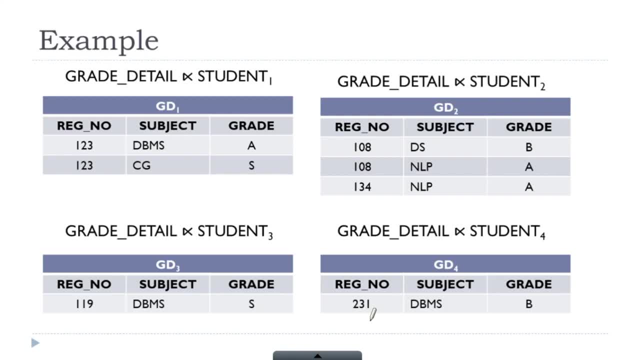 and grade detail 2, the register number 1,, 2,, 3 is the only student who end up in fragment 1.. Likewise in grade detail 2, that is, grade detail 2, what we have is 108 and 134.. So 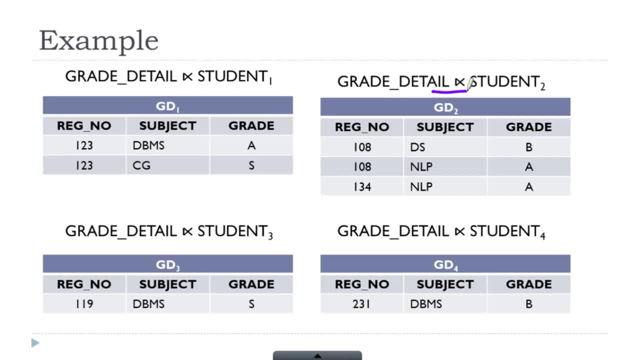 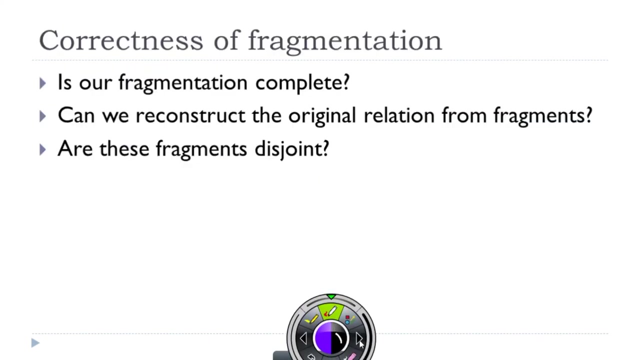 these two students are part of student 2 fragment. Likewise, we have fragmented into 4 fragments, 4 fragments. Now the related details are end up in same site, So one particular site all these records are end up in. So this is what the derived horizontal fragmentation. 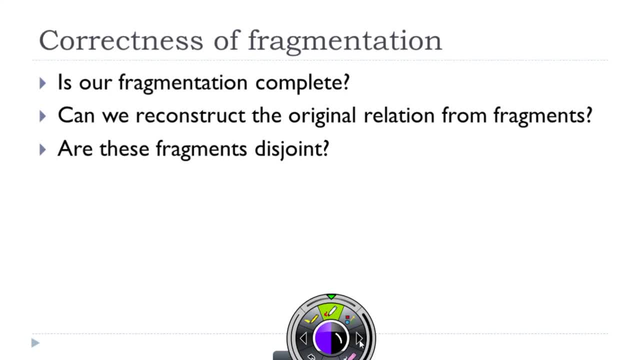 is about. So, once we finish this one, there is an important step that is correctness of fragmentation. So this is very, very important, that is, it is to check whether we have missed any data during fragmentation or any data is added extra, So that we want to be careful about. 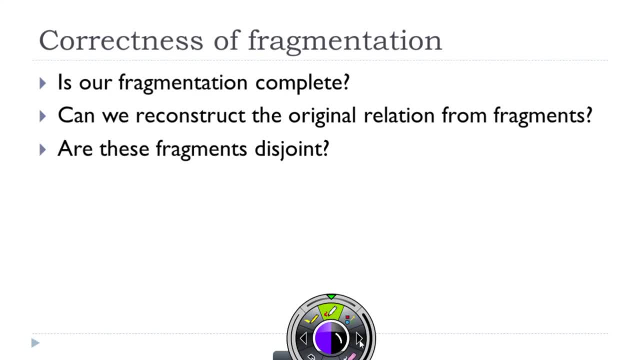 this. So correctness of fragmentation. the first one is: is our fragmentation? So we have checked the everyday: is our fragmentation is complete or not? So how do we check that? Are we missing any data? So that data should be available, that data of grade detail should. 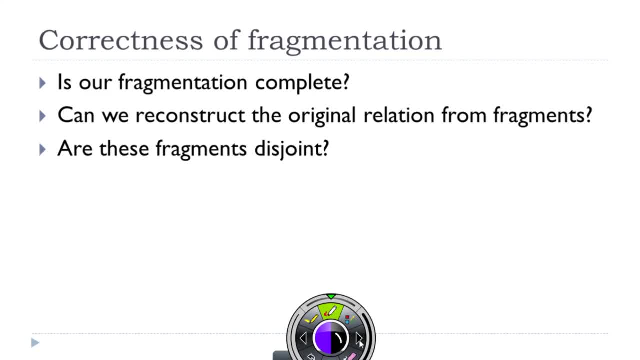 present in any one of these fragments. at least it must be a part of any one of these fragments. That is why the first rule is about The second rule – can be: reconstruct the original relation from fragments That is I perform. joining of, that is, union of all these fragments. I will end up in the original. 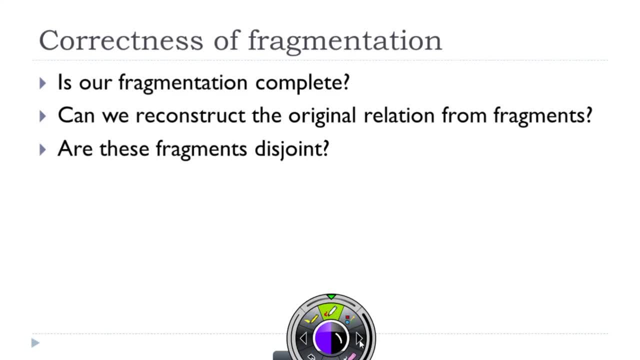 grade detailed table. And the third rule, that is theTHE frontier it has set here. that is engineering, how to make languages. one phrase inter еn f. All I have to do lies this one. And the third condition is: are these fragments disjoint? So disjoint is a property that 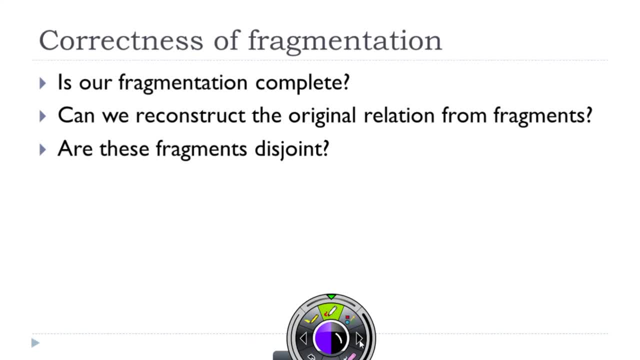 ensures there is no redundancy exists in a while fragmenting the relation. While fragmenting the relation, we want to be careful about no record should be part of more than one fragment. So that is, we want to find: are these fragments or disjoint? So if you perform, 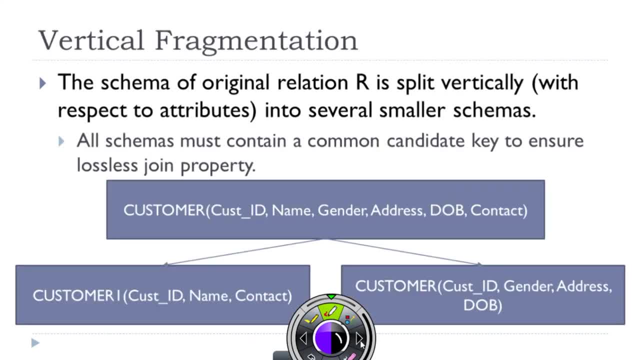 intersection between all these tables, we will end up in no record for common Vertical fragmentation. the next concept is vertical fragmentation. So I already we have finished with the horizontal fragmentation, where we have discussed about two varieties: One is about primary horizontal fragmentation, the other one is about derived horizontal. 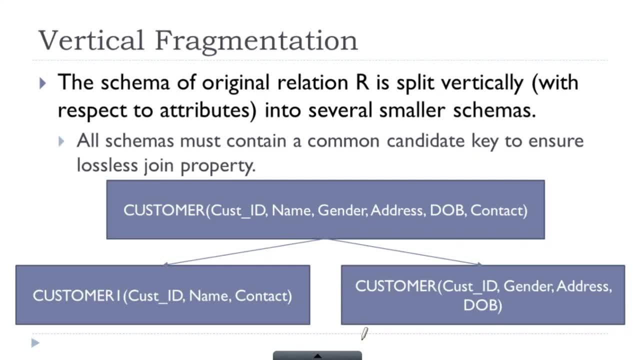 fragmentation. Now the next one is vertical fragmentation. So we are going to discuss about a little bit about vertical fragmentation, not too much about this. So vertical fragmentation is a way of decomposing a table into two or more tables. It is a simple a way of decomposing a table into two or more tables. Why do you want to? 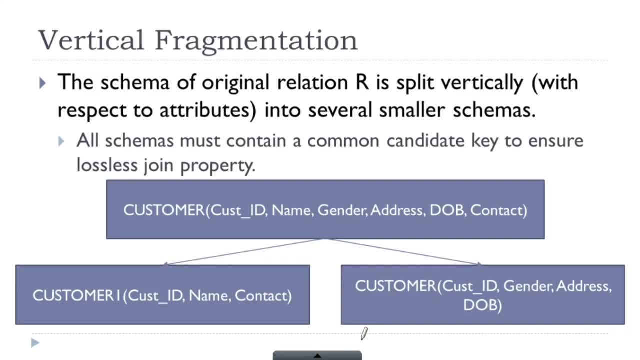 do that. In some cases we have a big table. The big table, not all the columns of these big tables, not all the attributes of this big table, is needed in all the different sites that we have in a distributed database system. We may have something like one portion of. 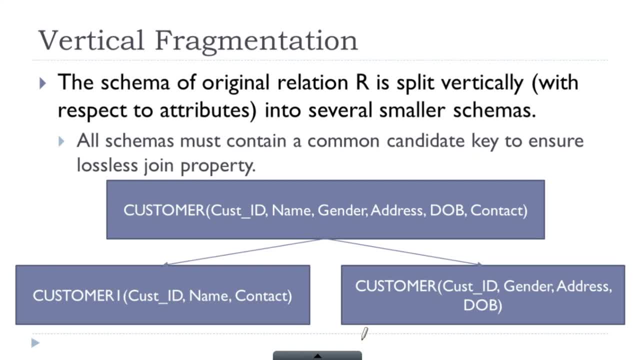 this table. Okay, If one person is interested in all the sites, one portion may be very much interested to only one particular site. That is in such case I want to fragment my table vertically so that I can place the part which is common for all in one location which is unique for. 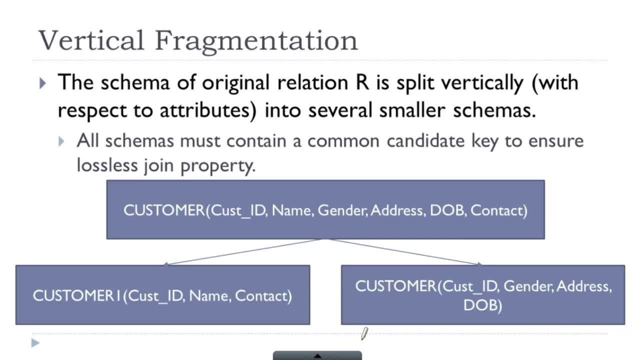 each site at each different sites. That is what we want to do. That is why we use vertical fragmentation, And it is just like the process of vertical fragmentation. it is decomposition. decomposition, that is, during the normalization process, you must have studied decomposing. 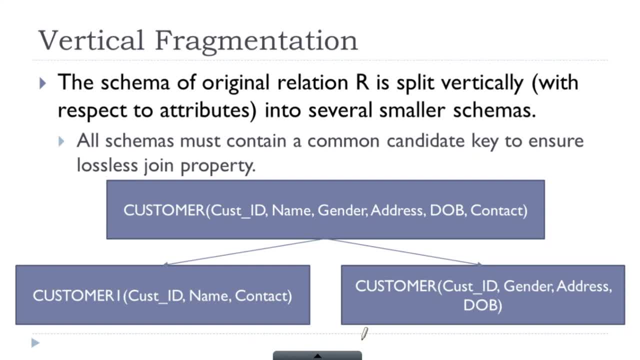 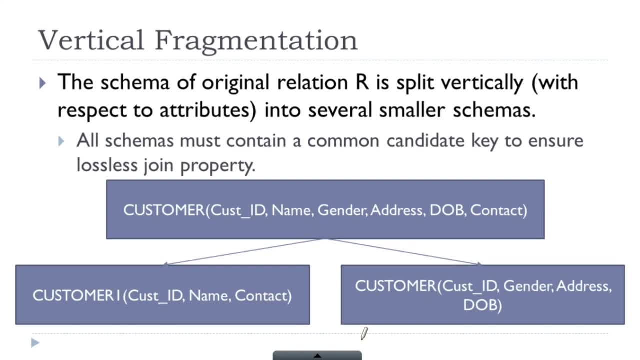 So all schemas- one property is. all schemas must contain a common candidate key to ensure lossless joint property. Lossless joint property. what is that? So during the decomposition we are going to break a table in such way that we want to retain the losslessness property. 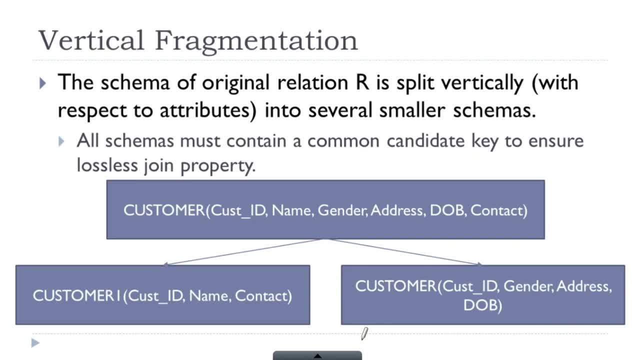 That is the reason why I break my table is to use it differently. So the way I break the table, the ways are: I may use the fragment, that is, one fragment alone, or I want to join these two relations back to get the original relations also. So there are different requirements. 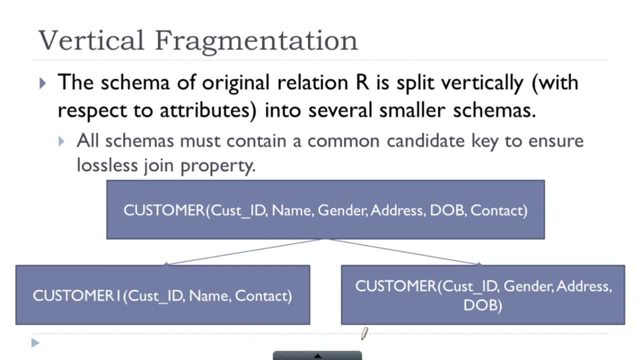 so that we must ensure the lossless joint property. That means I broke my relation into two or more relations. So when I perform join between, join operation between these fragmented relations, So I must end up in original relation without losing any information, any information that 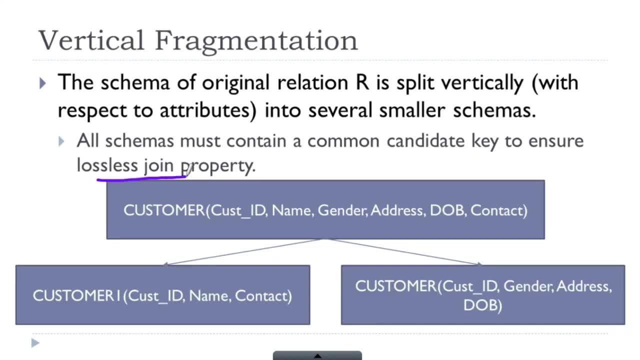 is what the lossless joint property is all about. See an example here. there is a customer relation with a schema: customer ID, name, gender, address, DOB and contact. Now we want to fragment this relation vertically. That means: 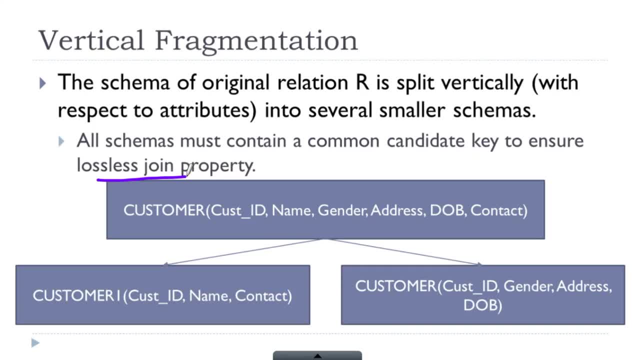 customer ID attribute, name attribute, contact attribute into one fragment And in another fragment custom gender address and DOB. gender address and DOB we want to break into into separate relation. The reason would be like this: gender address and DOB. 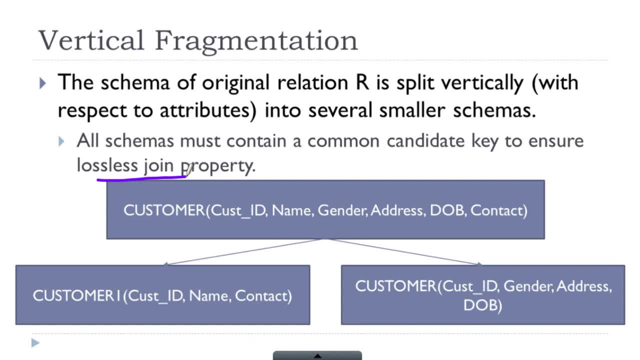 may not be frequently accessed by the application. On the other hand, customer ID, name and contact may be accessed frequently so that we want to place it in different locations according to our requirement. application requirement. Now, when I break this table, 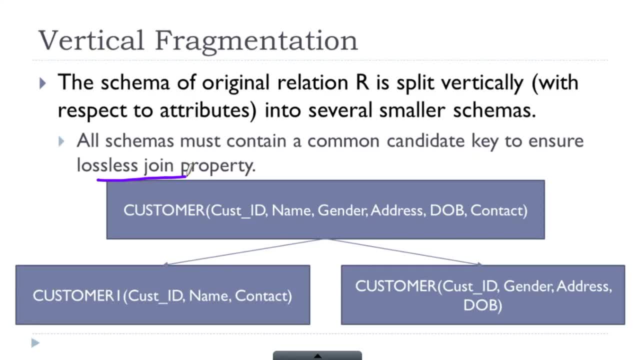 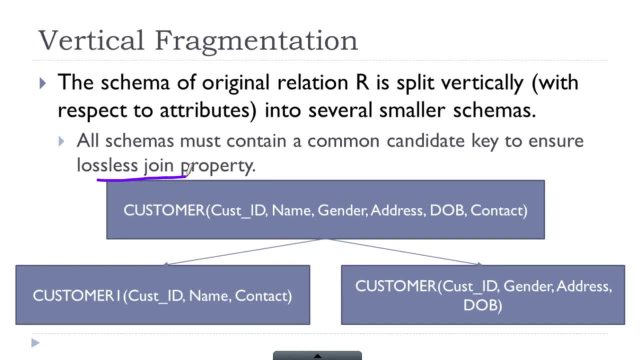 be a common candidate key, common candidate key. So what we have is here the customer ID is taken, which is the primary key of the table. This table is taken into both the fragmented relations. Now what we have is the vertical fragmentation of the relation customer. So 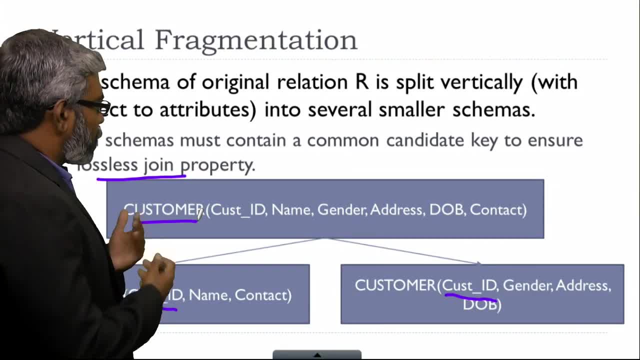 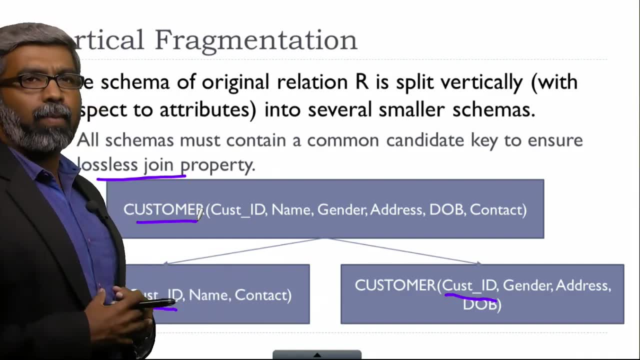 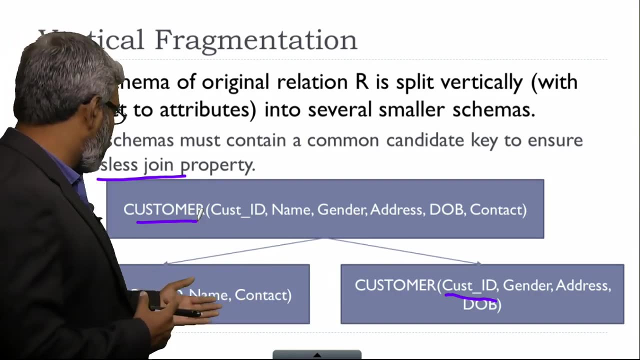 what we have is a very simple way, a very simple way of doing this one. I just want to break my relations into 2 or more relations, And it is based on the applications that are trying to access frequently. This portion may be accessed frequently. customer 1 may.